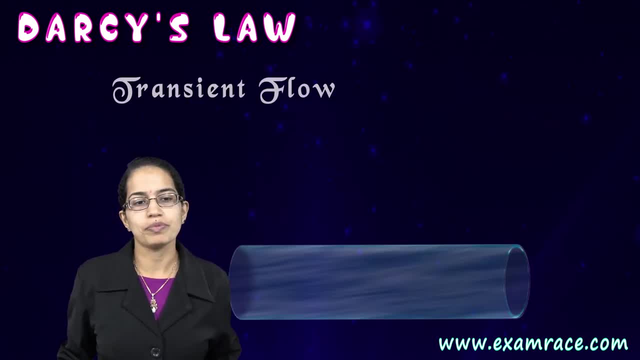 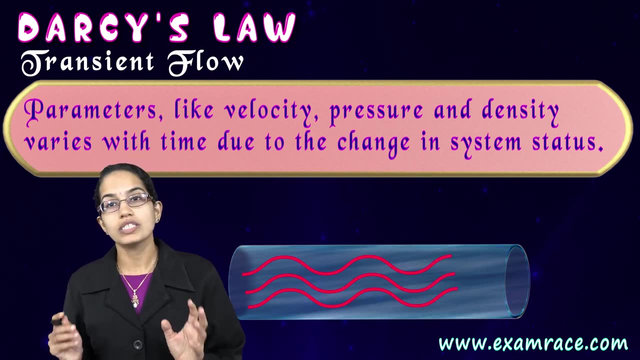 as a turbulent movement. And the third is a transient movement. Transient movement means these properties that we have discussed so far. they change with time due to the change in the status of the system and therefore we call it a transient flow. So whenever we 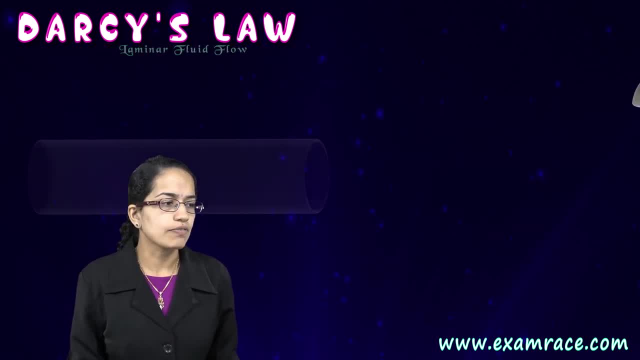 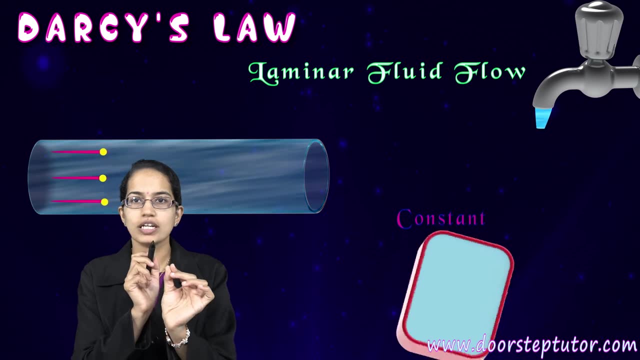 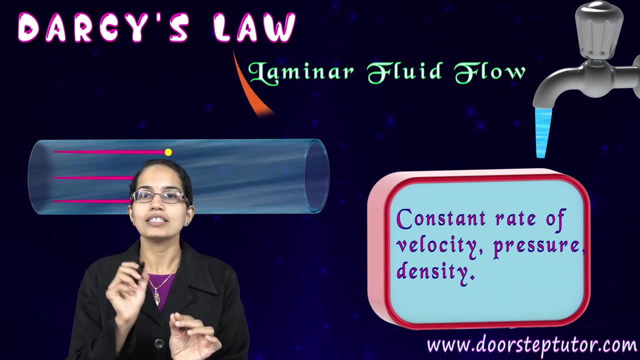 are considering Darcy's law. it's very, very important that we are focusing on a laminar fluid flow. So you have, at a given point, there is a constant rate of velocity, pressure or density that is seen. We call it a laminar fluid flow and Darcy's law is applicable in a laminar. 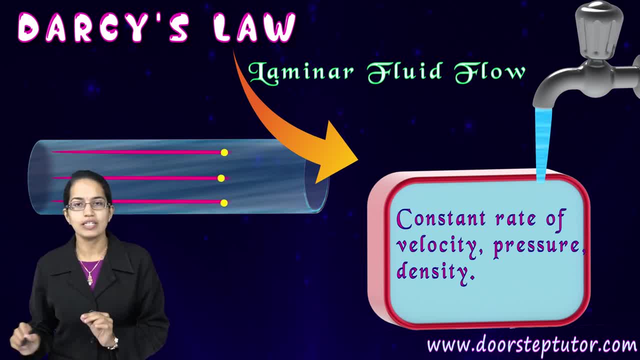 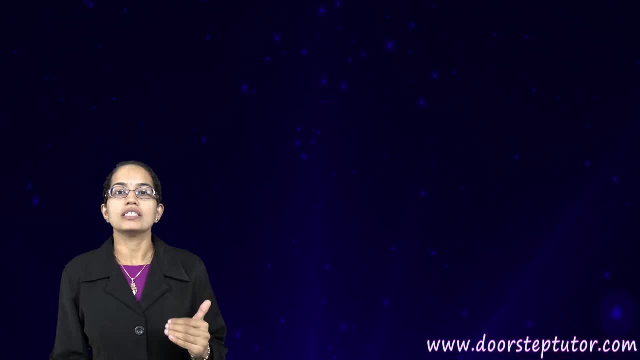 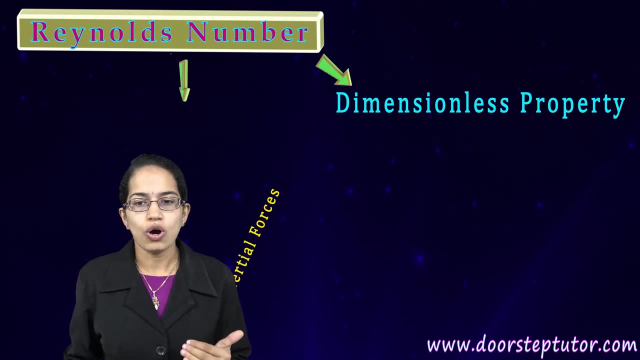 fluid flow, But there are certain exceptions that we would understand in a while. Now there is another important thing that we need to understand, which is the Reynolds number. Reynolds number is a dimensionless property. What do we mean by that? Reynolds number is the ratio of inertia to the viscous forces that are there, And this 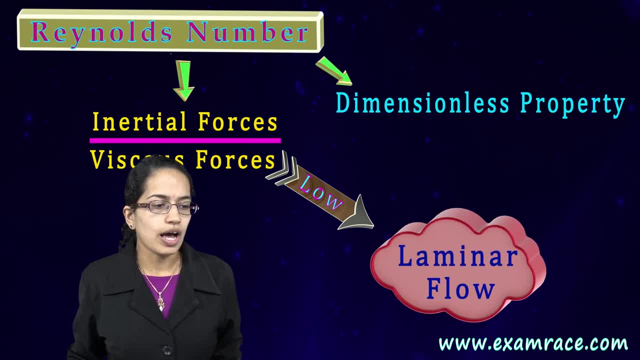 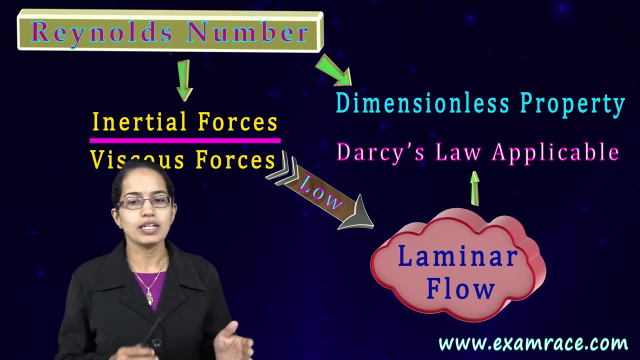 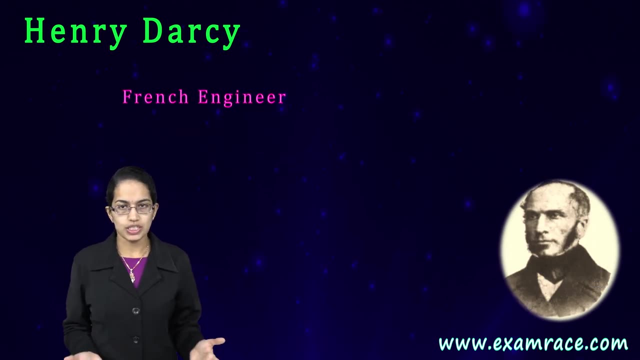 ratio. when it is low, we say that there is a laminar flow. So whenever you have a laminar flow with low Reynolds ratio, you would have the Darcy's law. that would be seen applicable. However, if this ratio is high, then it would be considered as a turbulent flow. Now Darcy. 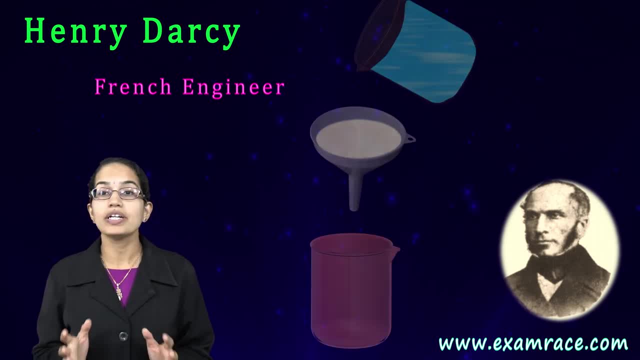 was a French engineer And what he tried to do was he used this principle to understand the mass of energy And the law of momentum And therefore we have this control of the pressure and the. the filtration- so sand filters- was the concept that he was trying to work on- and the rate of 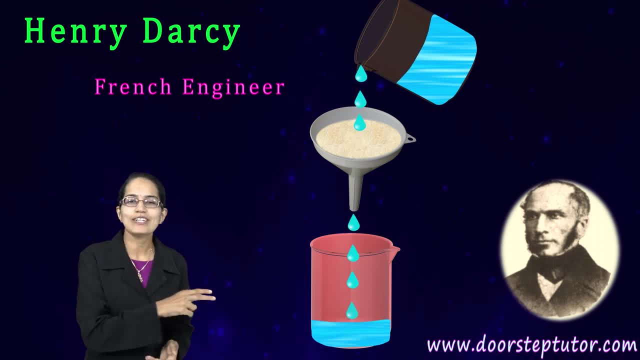 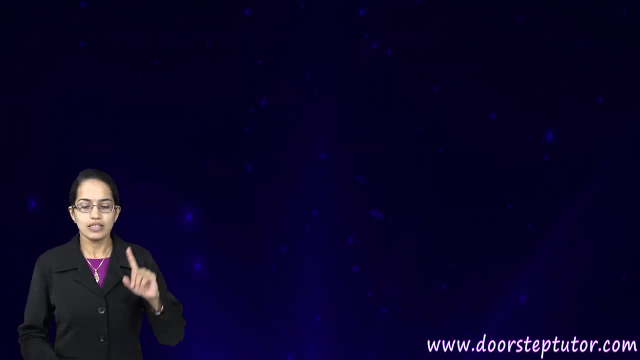 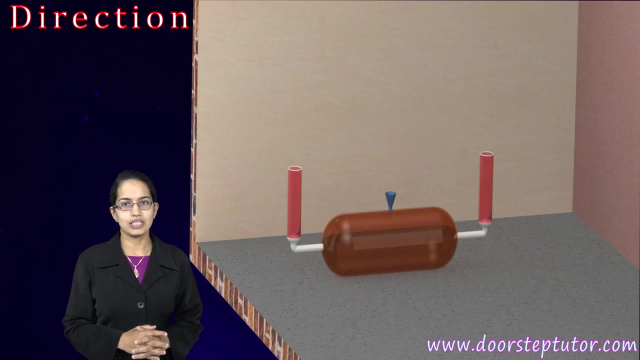 flow of water through those sand filters. but later on this law became highly applicable to ground water flow and there were two components that were seen. the one was the direction, the other was the amount of flow. to understand it, we have a very simple demonstration here. so we have a tank full. 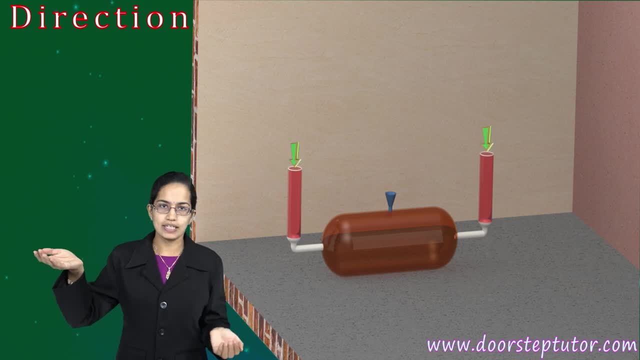 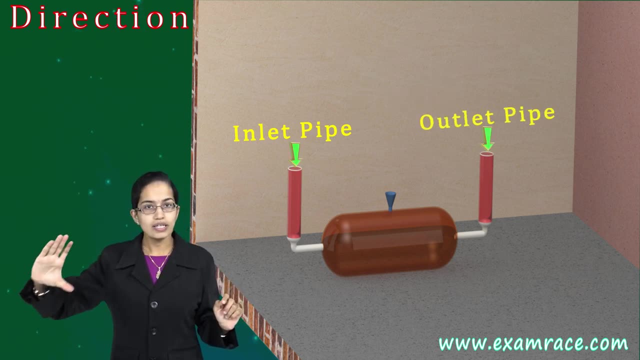 of sand, and then you have two pipes that are connecting it. one is the inlet pipe, the other is the outlet pipe. you have certain amount of water in the inlet pipe and certain amount of water in the outlet pipe. now what would be the direction of flow? that was the first problem that Darcy 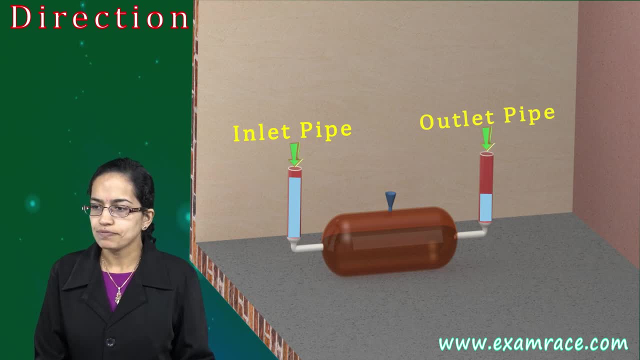 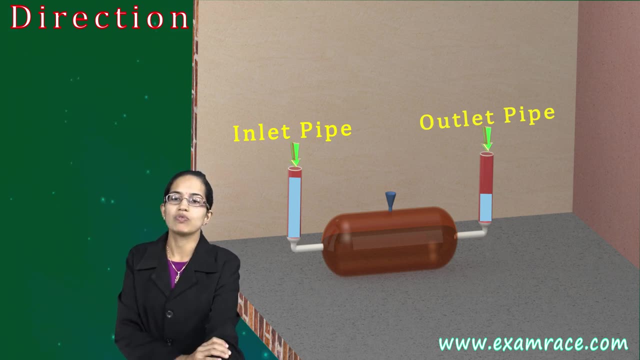 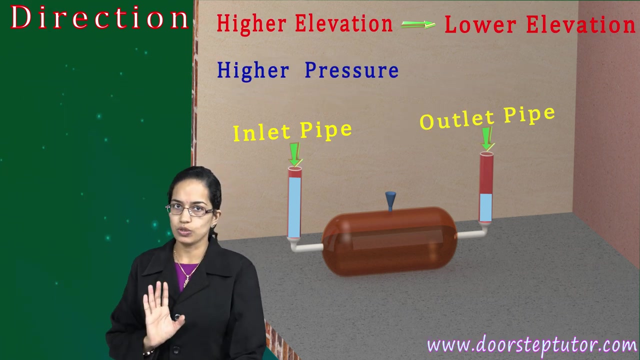 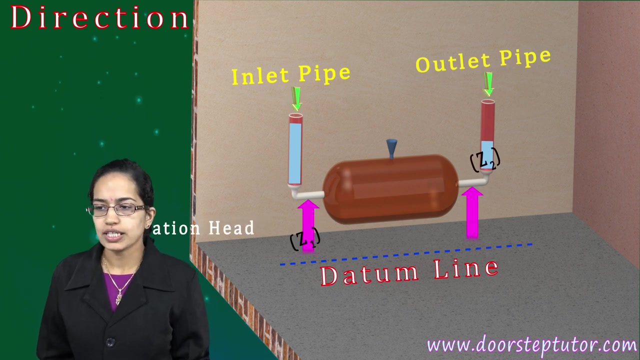 tried to solve. so it was simply, when you have a sand filter with the input and the output, a simple principle that works with water, as water flows from higher elevation to the lower elevation and from higher pressure to the lower pressure. so you had two components that were taken into account. one was the datum line and the elevation. 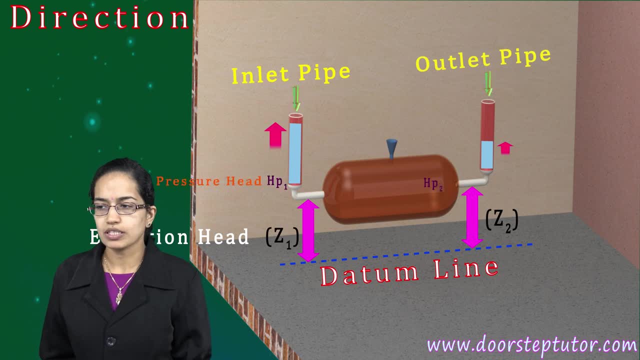 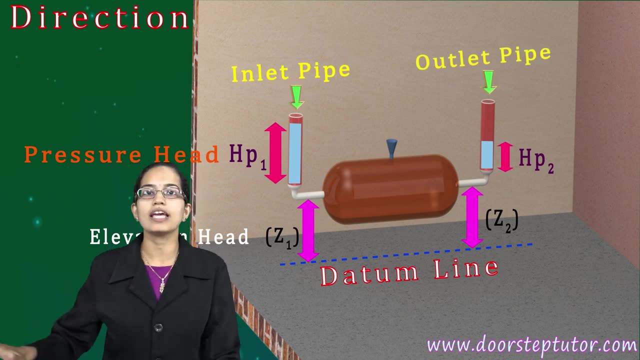 head. that was considered on both the sides, and then next was the pressure component that was taken into account. so let's say, the elevation component- component in the first case- remains same for the inlet as well as the outlet. so the only change would be seen with a pressure component and you would have a 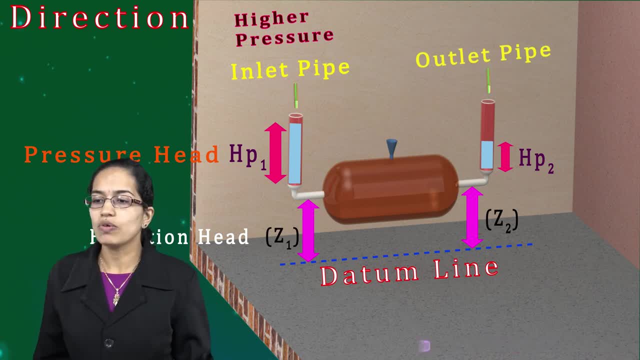 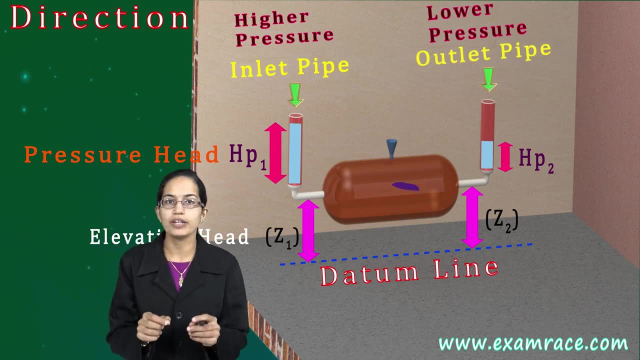 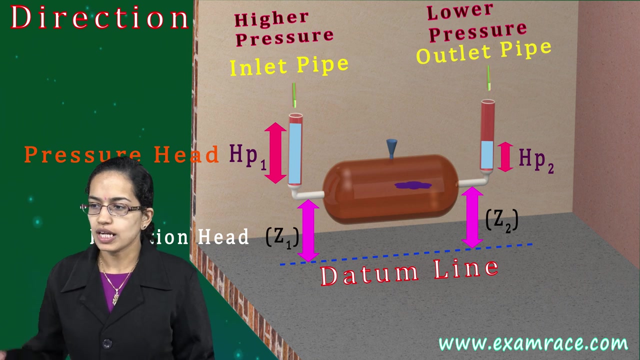 higher pressure pressure component with the inlet and lower pressure component at the outlet. so what would happen if I am trying to put a blue colored dye in the sand at this point? what would be the direction of the flow of that dye, since you have higher pressure and lower pressure, higher head gradient and lower? 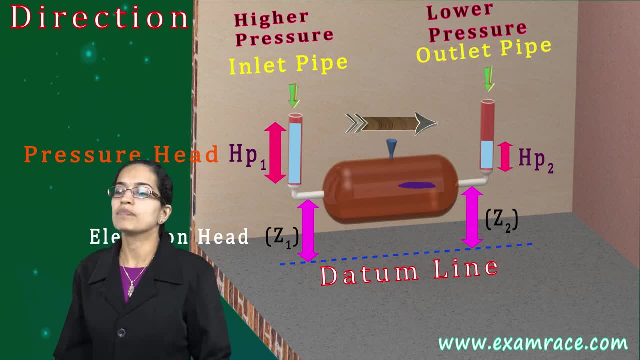 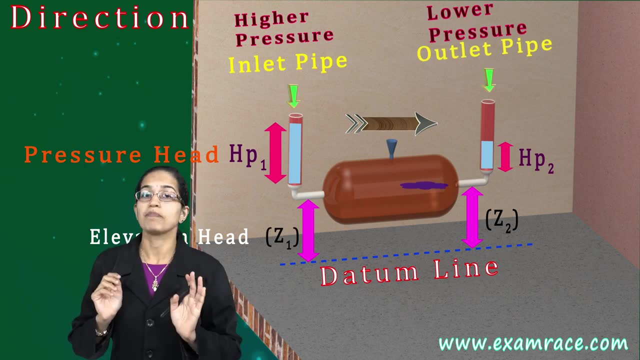 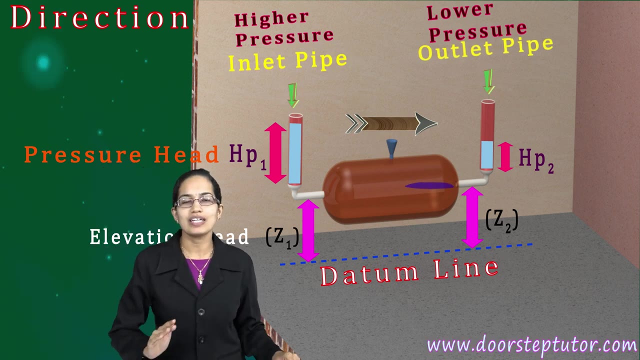 head gradient, you would have the movement that would be seen in this direction and therefore you would have the dye that would slowly and gradually start moving towards this direction, and this is how we understand the direction. so this was the first and the very simple case. now what I do is a 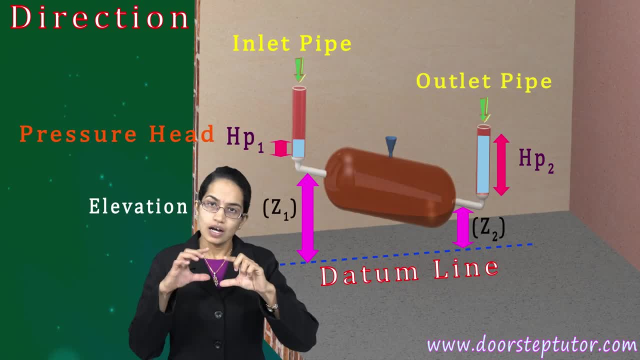 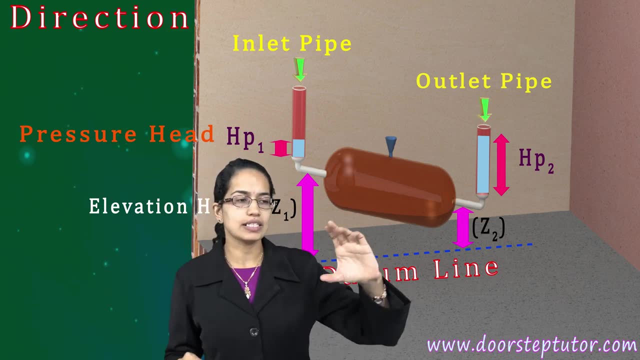 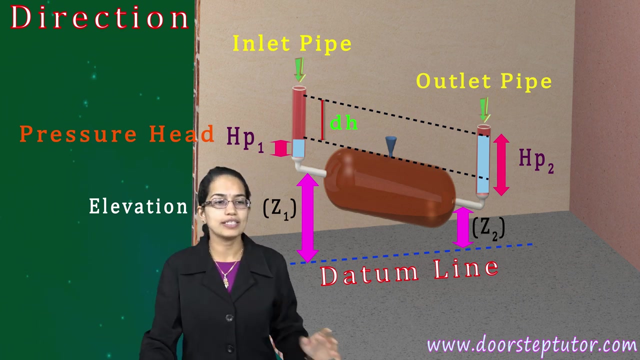 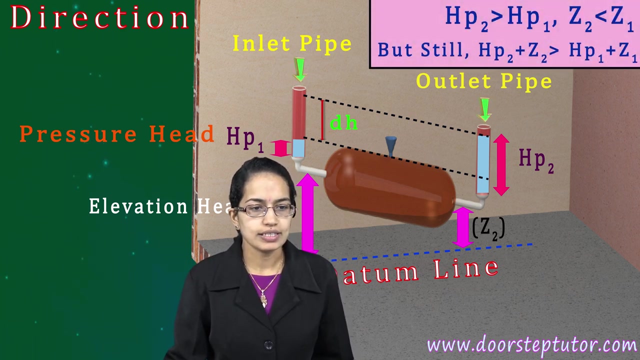 little interesting scenario where I tilt this sand tank. and when I am tilting this tank of sand, what is happening is I am again considering the elevation head and the pressure head. so together- note it's very, very important. let's say: this is the tilt that is seen. now, if you have the input that is higher than the output. 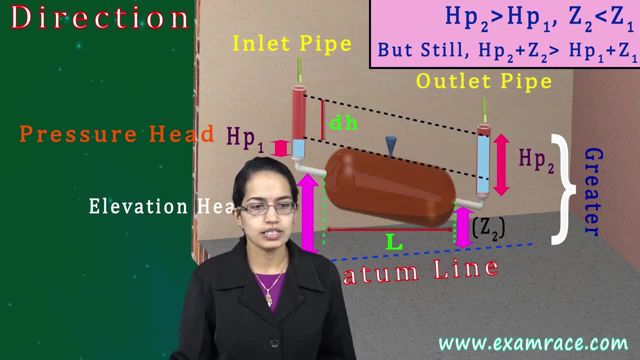 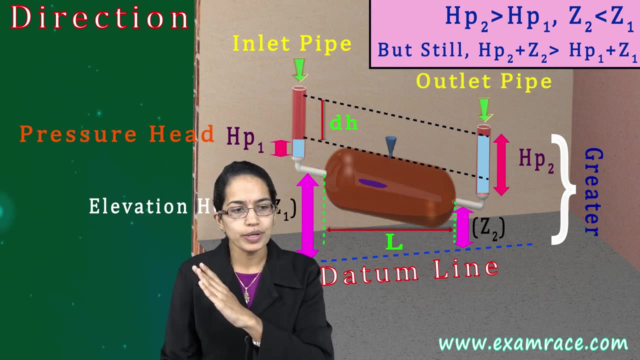 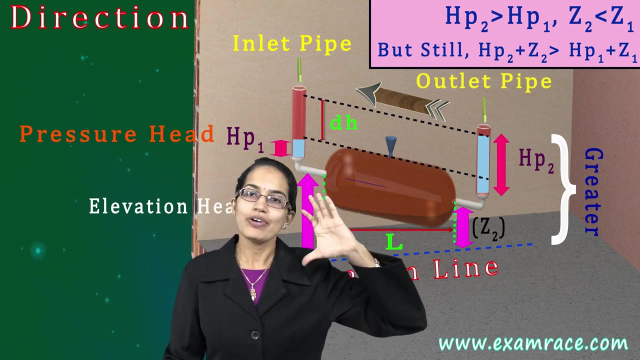 so my input is this point and output is this point. so always, despite that, the slope is in this direction. for the sand tank, the movement of the water or the direction of the flow would be opposite to it in this scenario, because you have higher pressure gradient and higher head gradient. that is seen in the output. 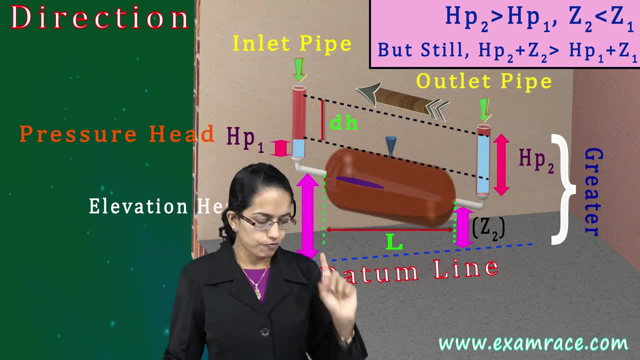 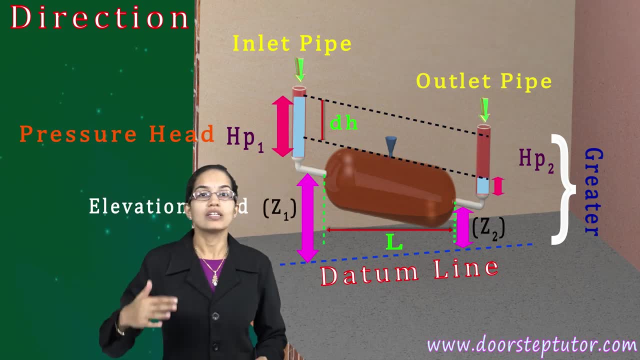 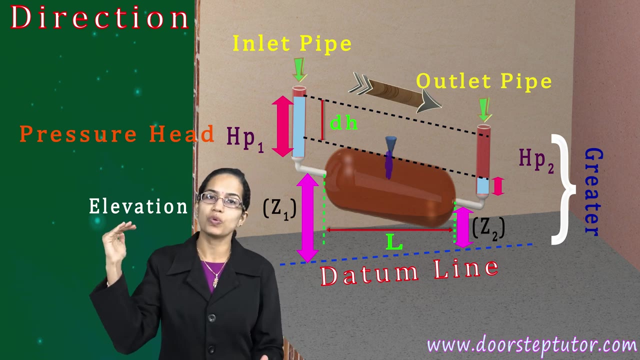 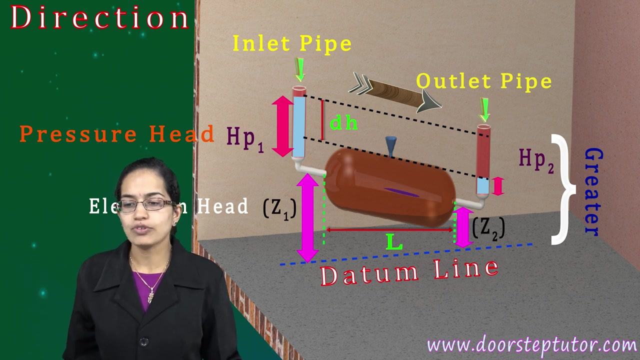 as compared to the inlet. so that is a very, very important component that you need to understand. however, it's good if you have both the slope of the tank and inlet proportion which is higher at the same direction, so you would have the smoother flow that would be seen in that direction. but ultimately, what you have. 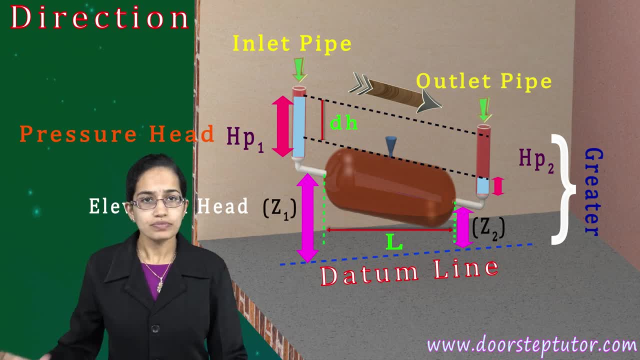 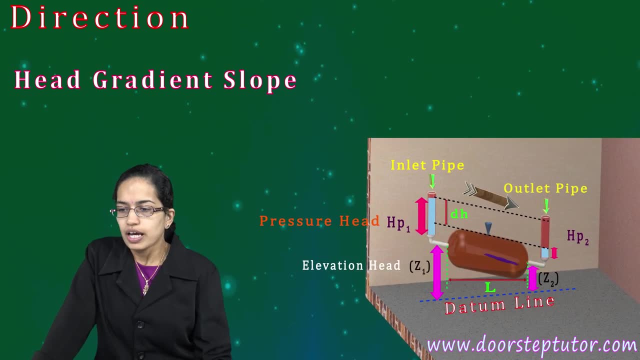 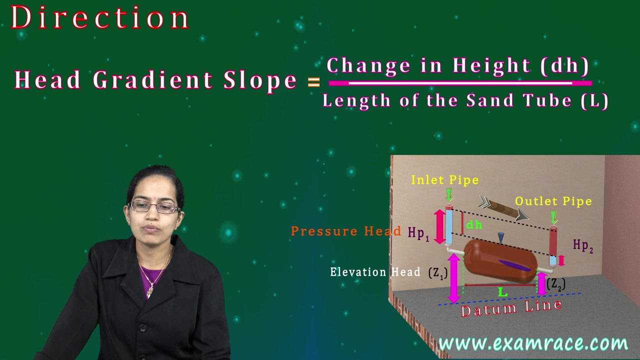 to understand is: is the higher amount of the total head gradient that we see? and this head gradient, how do we calculate? so we have what we call as the head gradient: is the change in the height divided by the length of the sand tube that is present, and this is something that we would be. 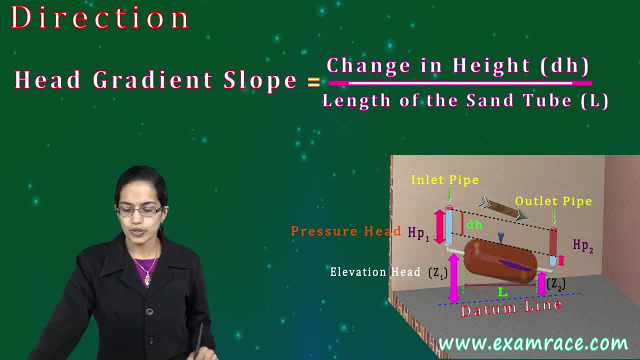 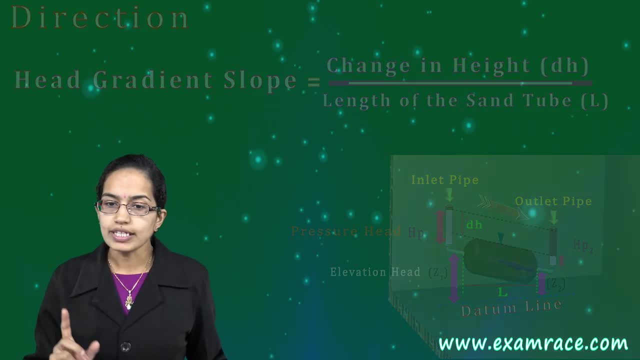 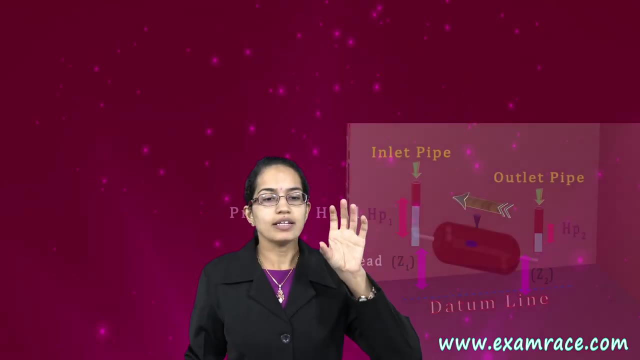 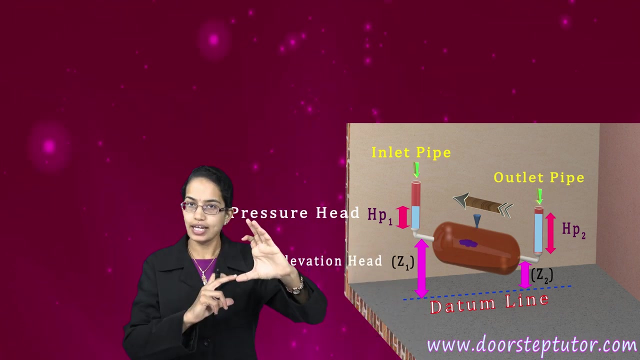 using later, when we would be talking about the amount of flow as well. so this is a very fundamental way to understand the direction of flow. the next important thing is flow. so, before proceeding to amount of flow, i repeat again, the most important point that you need to remember is you are trying to do changes with the pressure gradient and the elevation head. 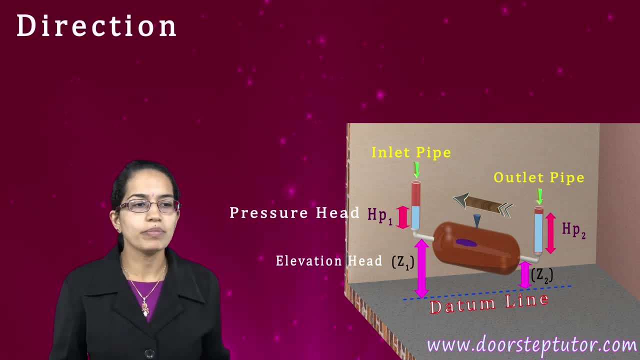 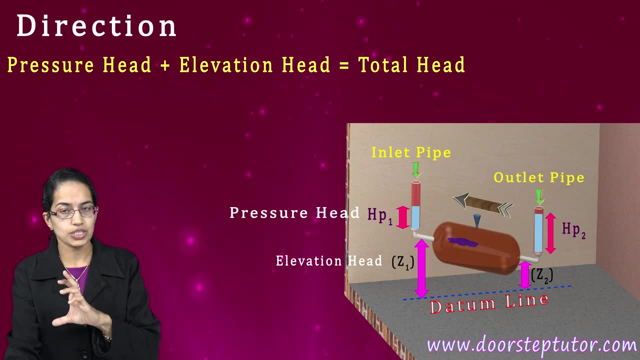 and whenever you are talking about the direction, it would be a combination of the pressure gradient as well as the head gradient. so together the pressure and the elevation would give you the total head and that would be the direction of flow. so ground water would flow from a higher. 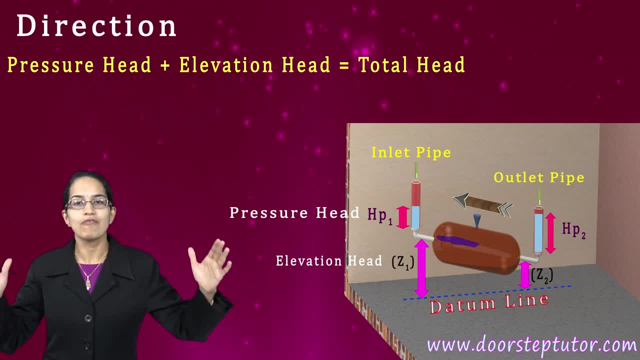 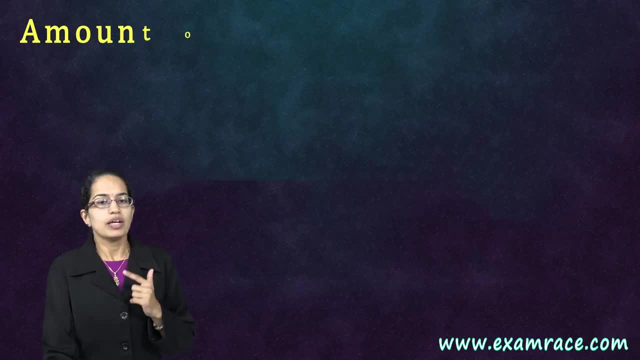 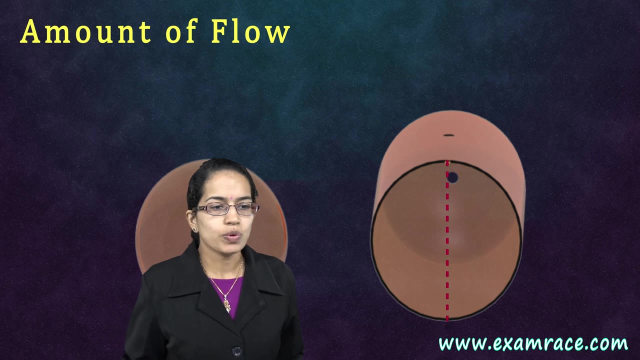 head to a lower head always, and this is a very simple experiment that we tried to demonstrate to help you understand. the next important is the amount of flow. now, when we are talking about about amount of flow, let's say the sand tank has this diameter, so you would have the water that 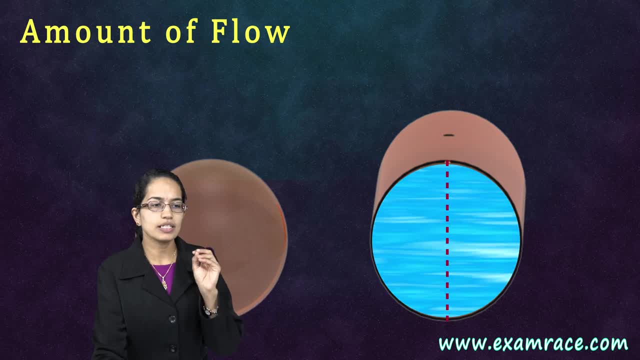 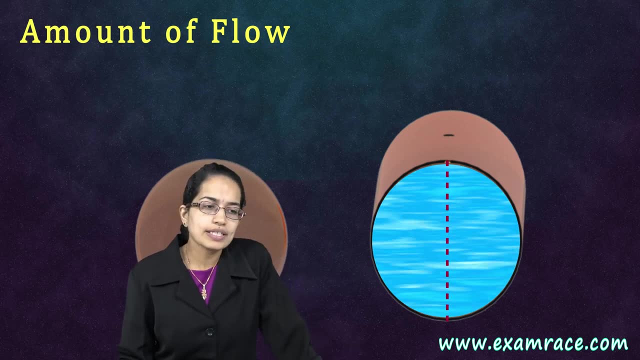 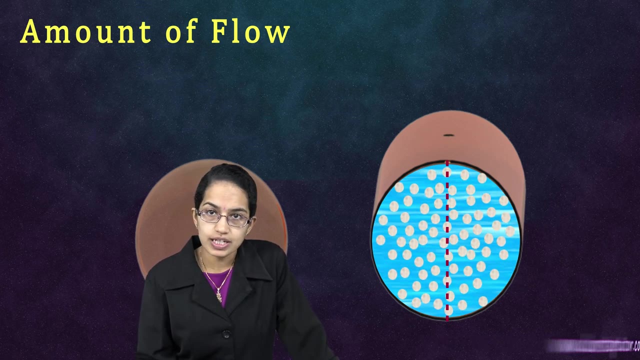 would flow through whole of this. now there is inter, there is nothing. it's open and it's a clear channel, so it would have a huge amount of water that would flow through it, but this channel, let's say, has intermittent scent particles. what would happen? you would have the area that would definitely change here and this change or, uh, the change. 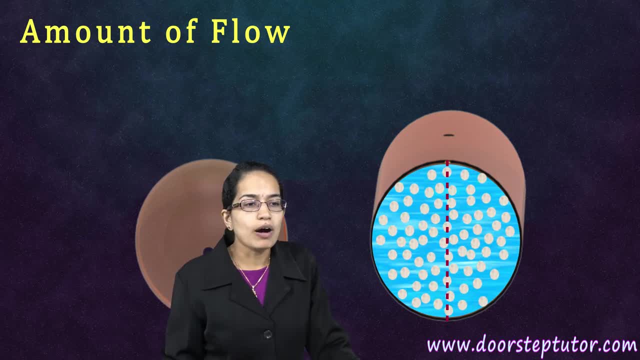 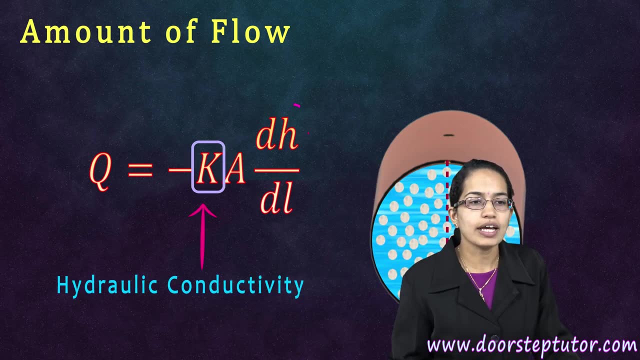 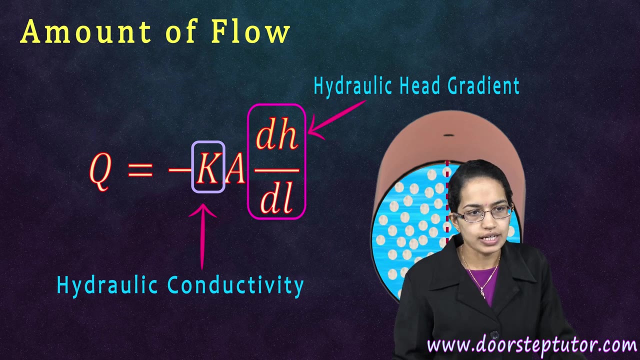 that would be seen would be affecting the amount of flow. so amount of flow, we say, is determined by a formula where we focus on the hydraulic conductivity and the head gradient- the hydraulic gradient, which is also known as the hydraulic head gradient- and the hydraulic conductivity and then the area. 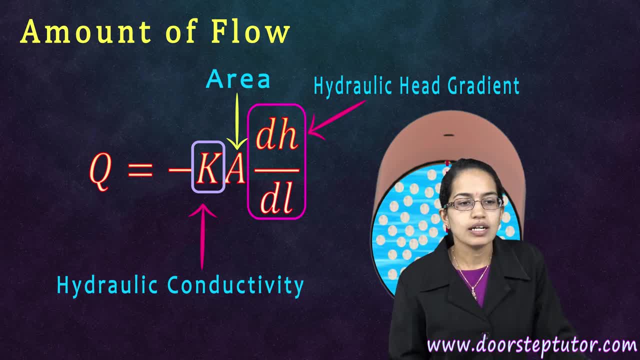 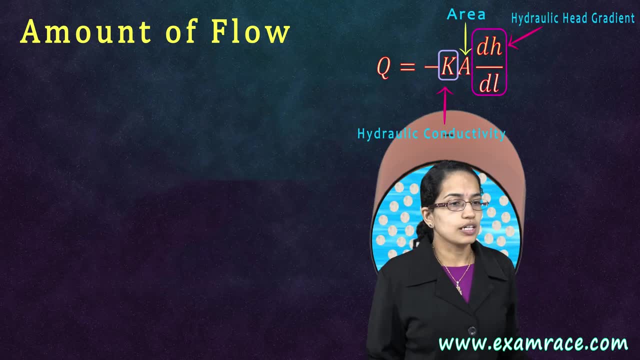 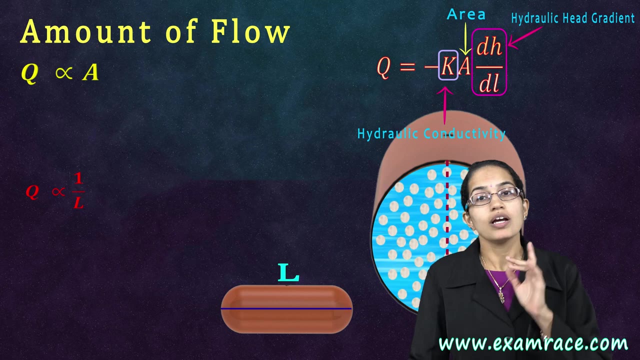 which is the diameter, which is considering taking the diameter of the channel through which it passes on. Before understanding this further, you have a simple relation: that the amount of flow would be directly proportional to the area through which it is flowing, but it would be inversely. 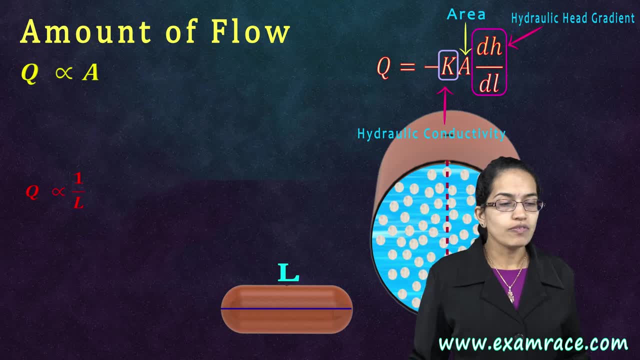 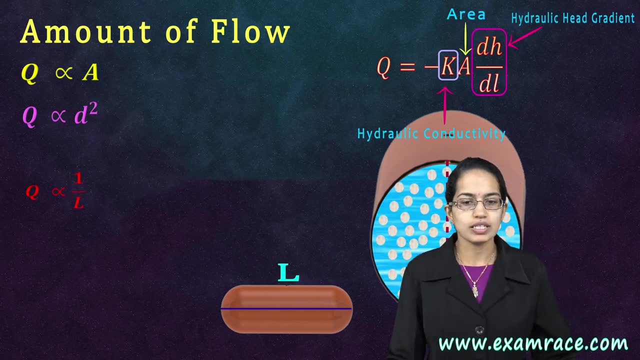 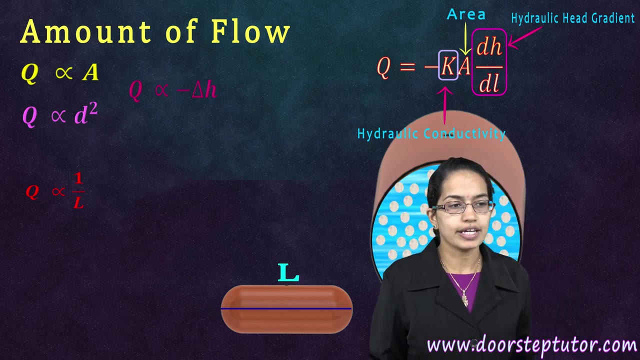 proportional to the length of the column that is there. however, it would be directly proportional to the square of the diameter, that's very, very true, or the square of the radius, that's true again. and it would be directly proportional to the difference in the head gradient. so the inlet 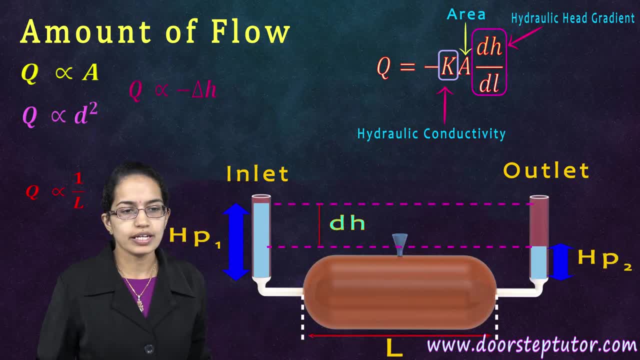 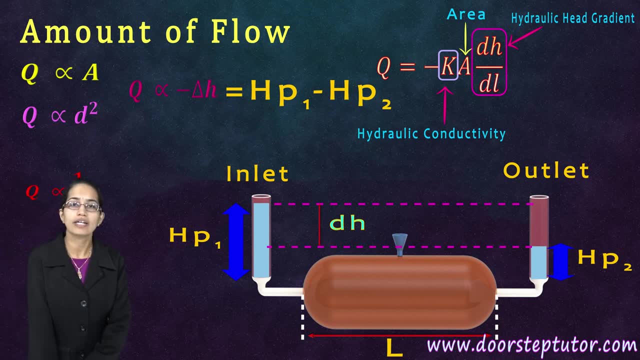 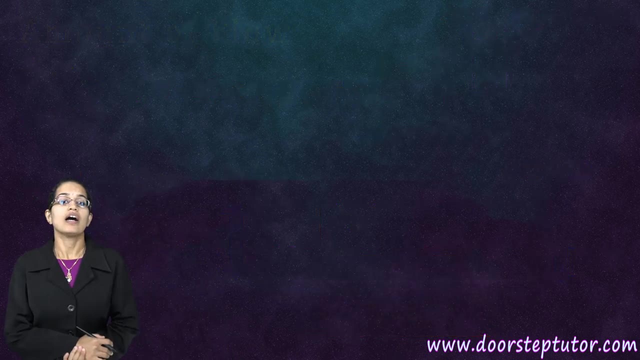 and the outlet being connected and the difference between the head gradient of the inlet and the outlet. so h1 minus h2 and that's the difference between the head gradient and that's where you have a direction relation with the amount of flow that is seen. but a very interesting thing comes up here is: 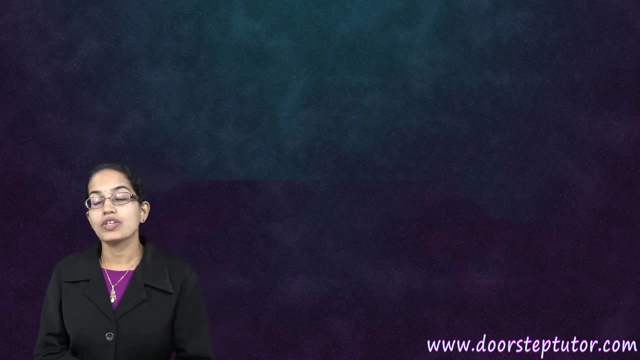 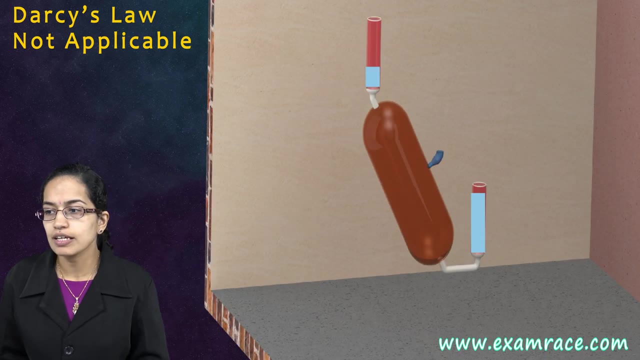 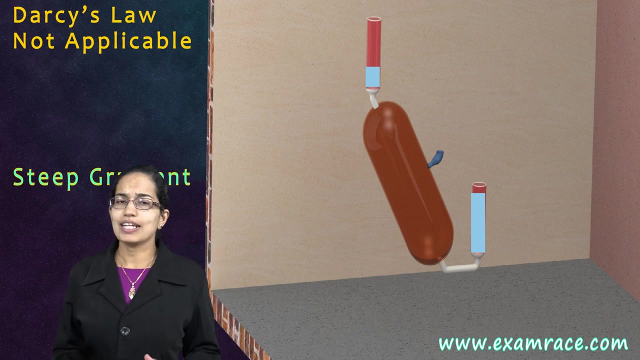 a question for you where i believe that what would happen if this head gradient is extremely steep? when this head gradient is extremely steep, what would be the situation now? you would be definitely, uh, by a kind of intuition. you can answer thus that when you have a very steep, 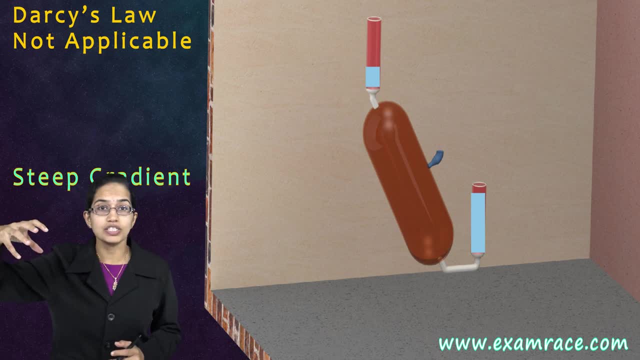 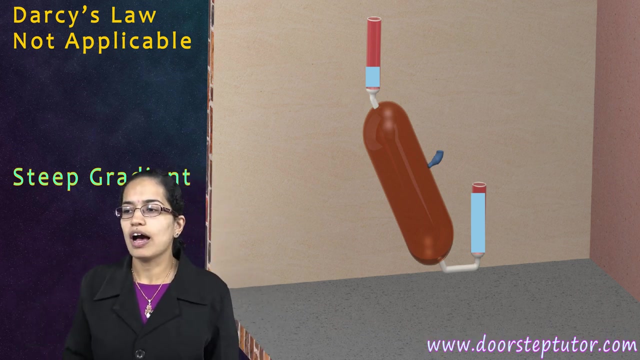 gradient. what would happen? the fluid would have enough energy to accelerate despite of any kind of resistance that is being provided by the particles of the sand that is present, and it would try to go downwards. but here is where you have inertia that comes into play. and since inertia comes, 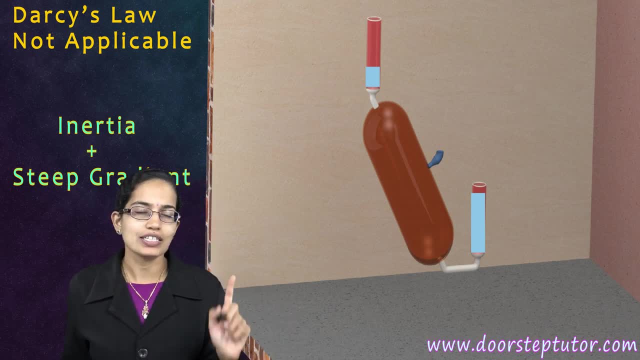 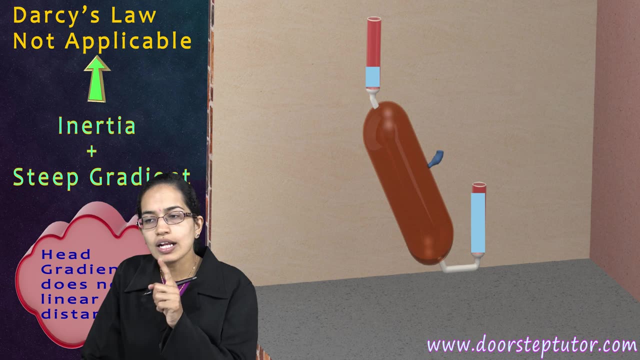 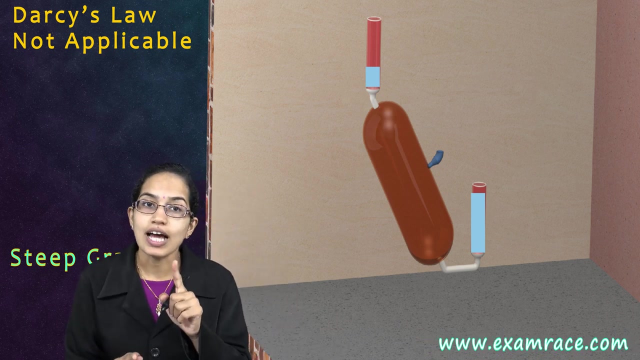 into play. in this scenario, you won't have Darcy's law. that would be applicable because the head gradient is not in a linear fashion or is not dissipating linearly with the distance that we can say. so whenever we can say that inertia becomes important, it's that the Darcy's law starts to fail, despite